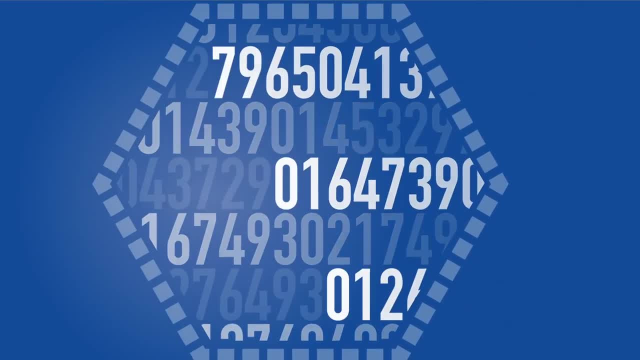 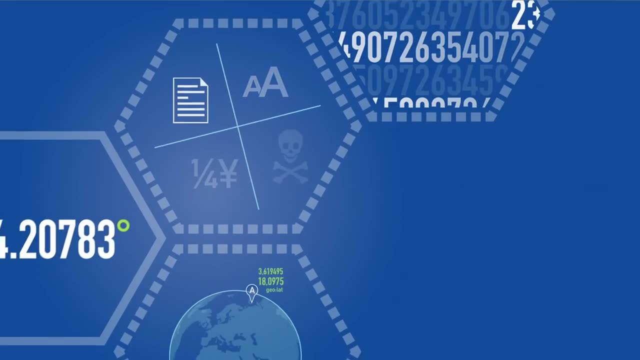 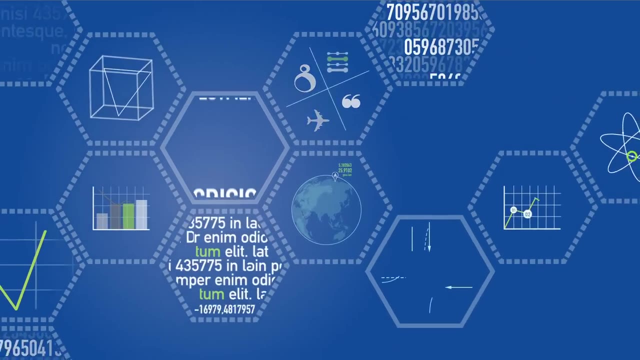 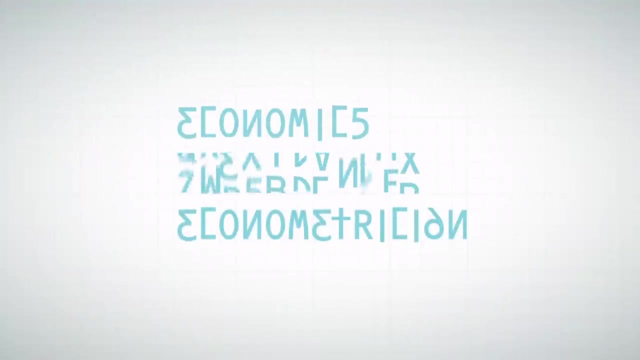 Worldwide, a storm of data is being generated every day, And every country, government, company or organization is in some way or other interested in this information because, if interpreted correctly by an econometrician, it can help to predict future interests. An econometrician is someone who is interested in and knows about, economic models, but he also knows his math. 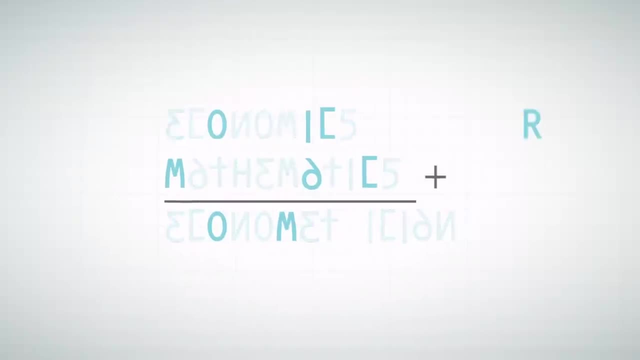 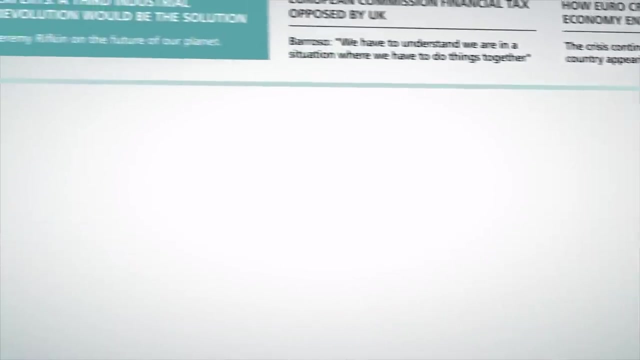 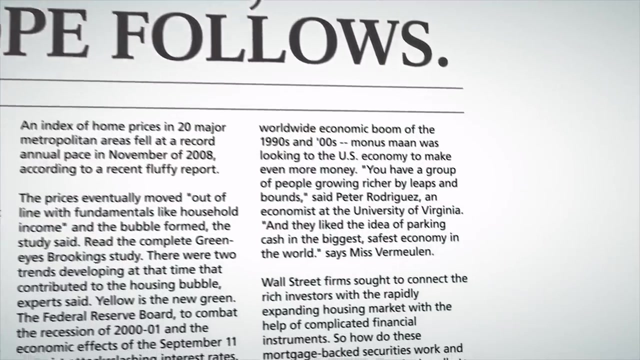 He likes to solve puzzles within the landscape of economic variables, both on a macro- and microeconomic level. For instance, a few years ago, when some big banks in the US crashed, many of the primary economic indicators went down. The US entered a major recession and Europe soon followed. As a result, countries in the European Union face many serious challenges. 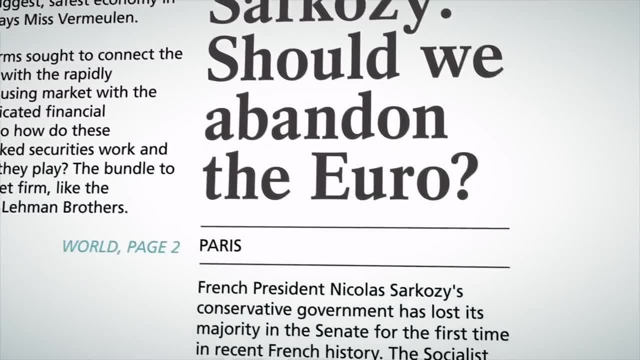 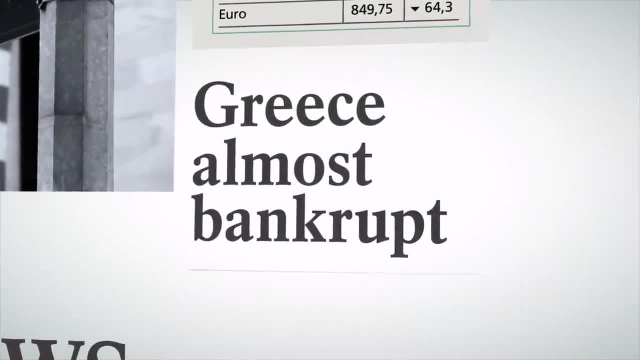 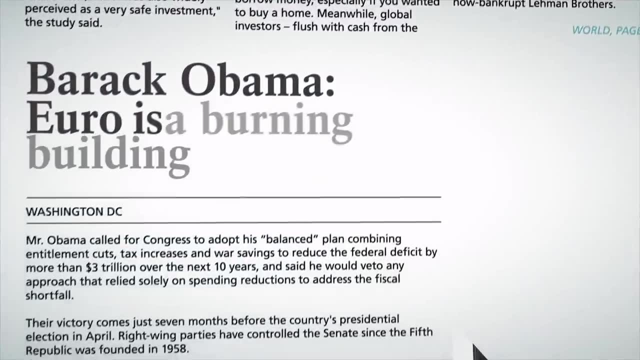 Should we abandon the Euro or should we keep it? Should we grant extra credit loans to Greece? Should we bail out investment banks or let them go bankrupt as a result of their own choices in the past? Often, politicians have clear opinions on these issues and present these opinions loud and clear. 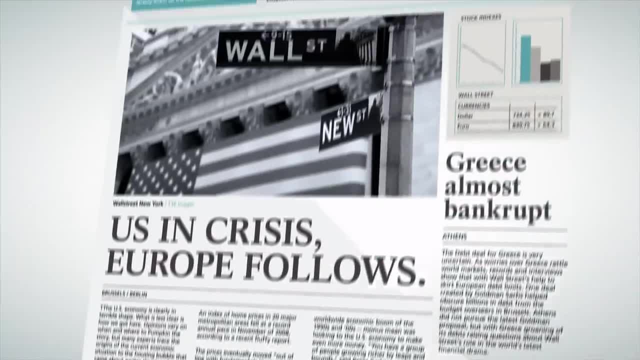 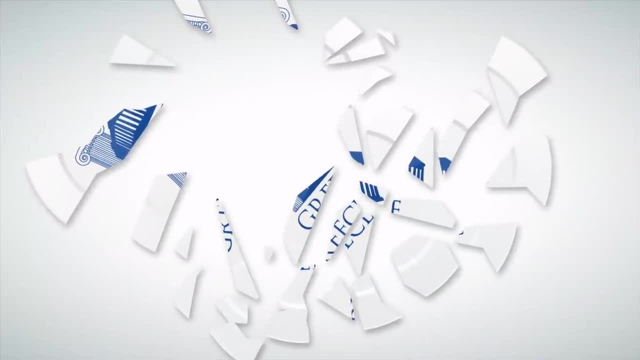 An econometrician, on the other hand, will try to predict the consequences of abandoning the Euro- or Greece for that matter, And he will also try to predict what will happen. if we don't, Then you and politicians will help him. 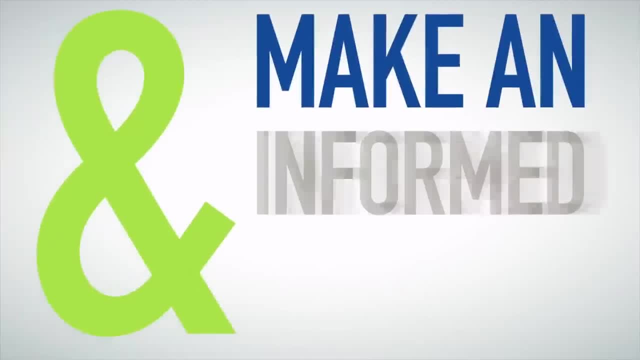 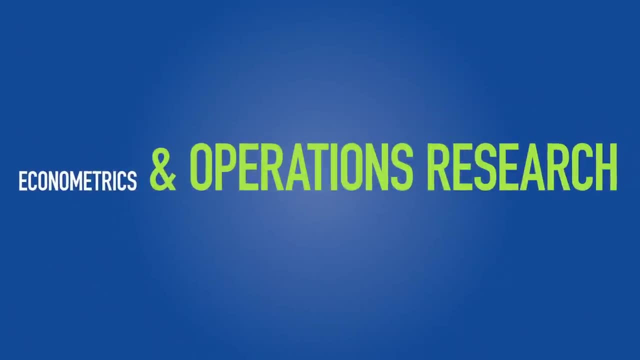 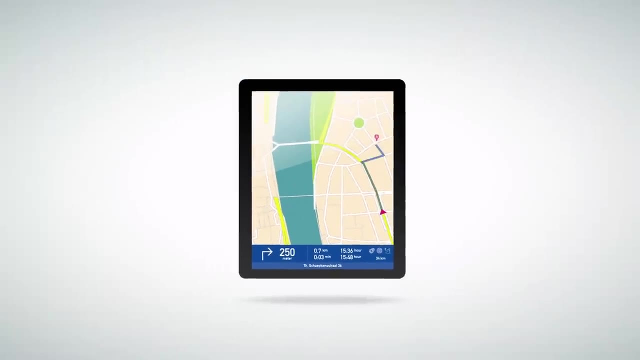 Politicians, too, can base opinions on facts and make an informed decision. Econometrics and operations research are also used on a smaller scale, influencing your daily life. These techniques are used to set up logistics systems or to determine how many people are needed in a call center. 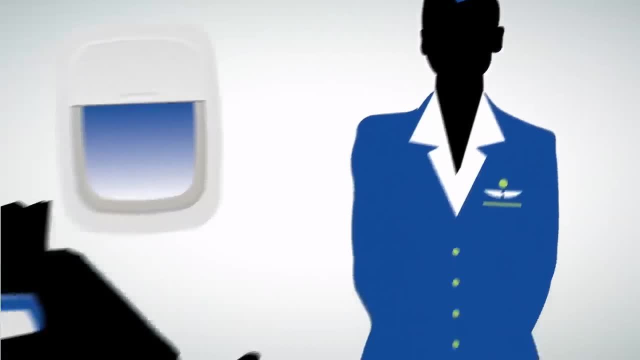 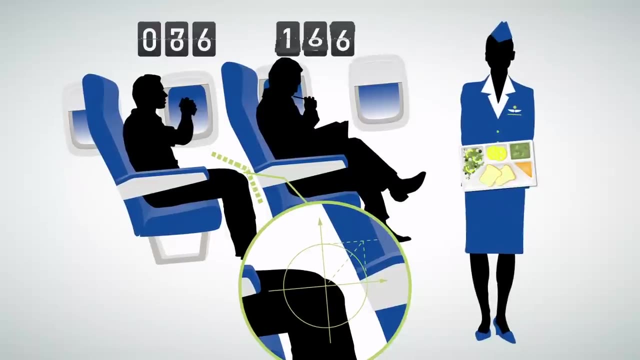 They can also set the price of an airline ticket. Did you ever sit in an airplane and wonder why the person next to you with the same amount of leg space and the same onboard lunch paid half the price you did? Econometricians know why. 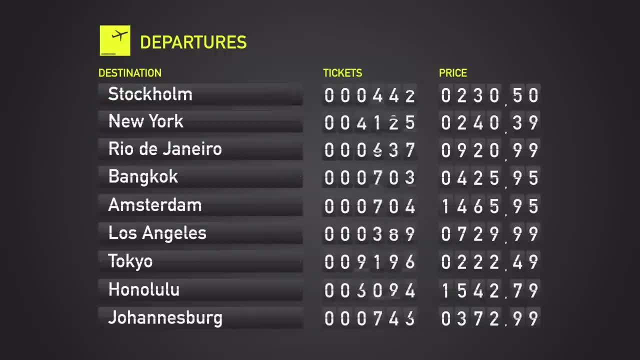 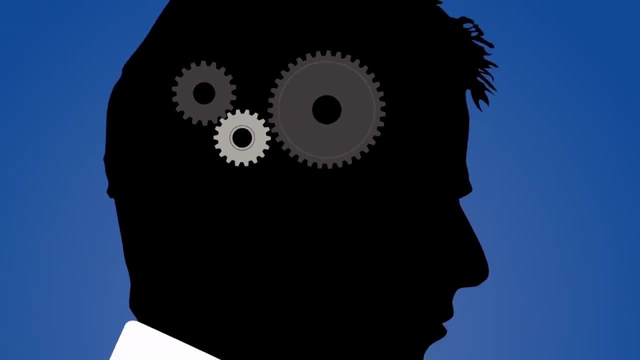 Electronic ticket reservation services register how many tickets are sold each day for each flight. When you raise the price of a ticket on a particular day, you will sell fewer tickets but for a higher price. Techniques from econometrics and operations research help airline operators to fine-tune their strategies.